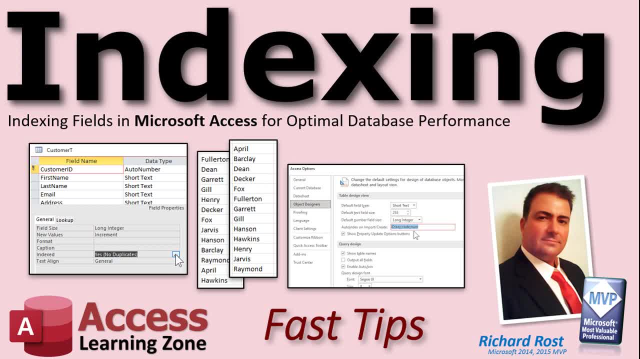 Actually, I just had to look that up. I just Googled that and there is a difference between Optimum and Optimal. I always just thought it was a matter of preference, Because Optimal is an adjective- For example, Optimal Performance- Whereas Optimum is a noun. For example, a properly indexed table is the Optimum for database performance. 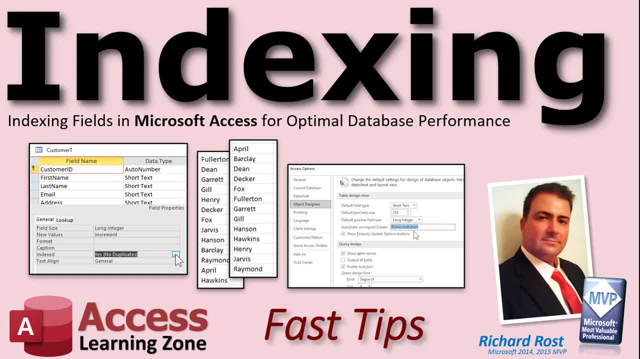 So I try to learn something new every day, And every time I put one of these videos together, I do a little research And I always learn some new tidbit that I didn't know before, So I love sharing this stuff with you guys. Alright, let's talk about indexing. 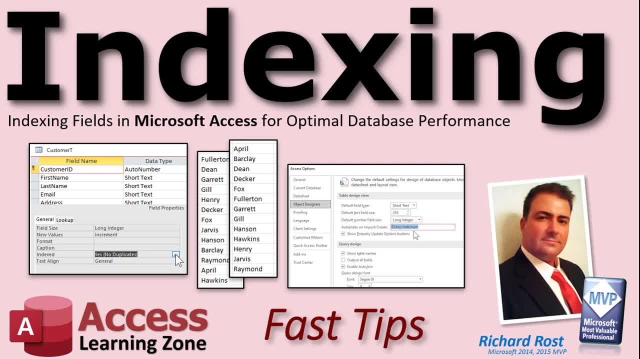 So indexing is one of those fields. Indexing is one of those features that is almost never used correctly by new users. You can get away without indexing anything at all in a small database. However, as your database grows, you're going to want to keep things running smoothly. 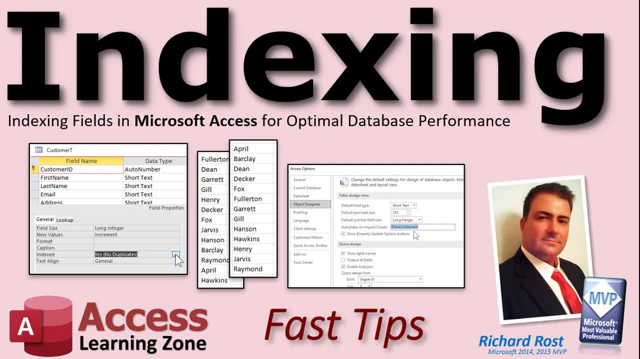 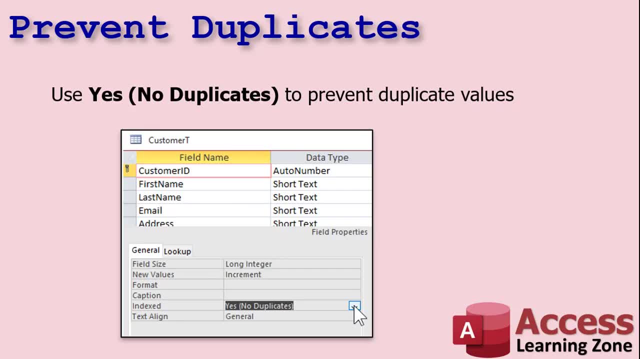 As your database gets bigger and bigger, it's going to get slower and slower, Especially if your tables aren't properly indexed. So the first use of indexing is to prevent duplicate values. This happens, for example, with an auto number. Obviously you want to make sure your primary key 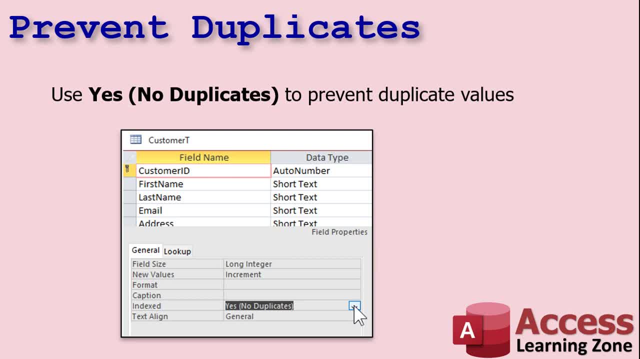 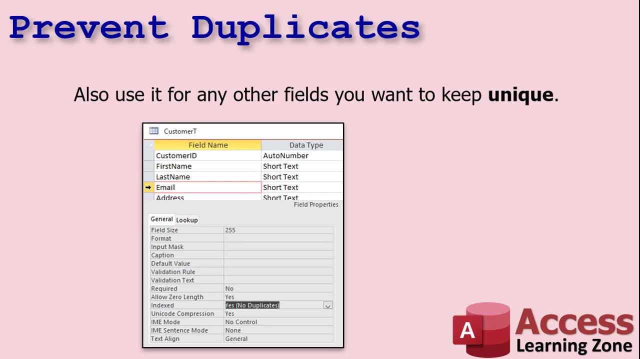 is indexed, so you don't have two customers with customer ID 3,, for example. You may also want to use indexing for any field you want to uniquely identify a record with. For example, I index email address as no duplicates. There can be only one. 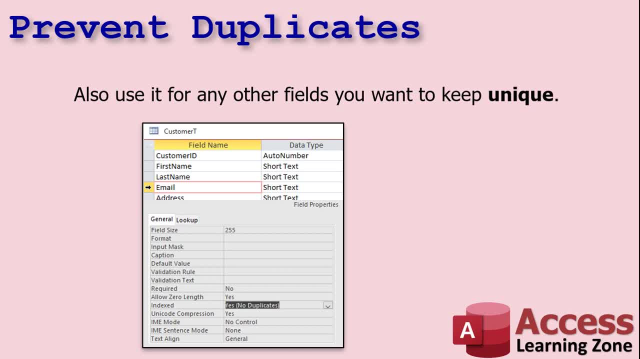 There can be only one right. There can be only one customer. That's amicron at gmailcom. That's how I look up customers in my database. If you try to type in another person with the same email address, you'll get an error message. 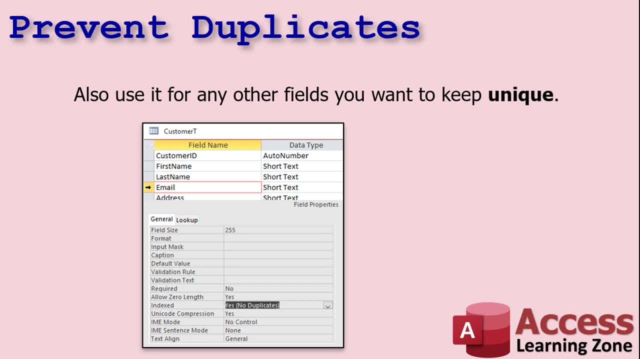 Some other companies I've seen use phone number to uniquely identify their customers, One of which I have a membership at, and every time you go buy something you get enough of a receipt to wallpaper your house with- And I'm not going to mention any names, but they ask for your phone number. 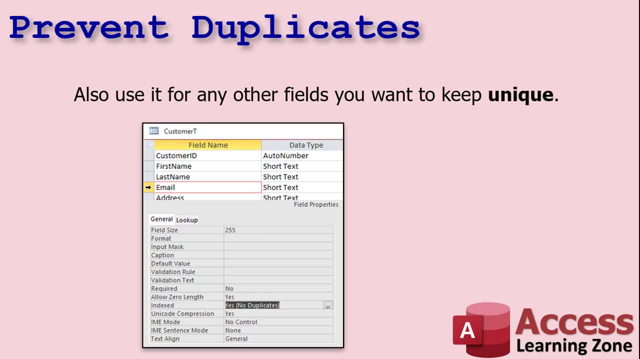 to give you your discount points, And that's probably an indexed field in their database, And if it's not, their IT department is slacking. Alright, so that's yes, no duplicates. Now you can use yes, duplicates, okay. 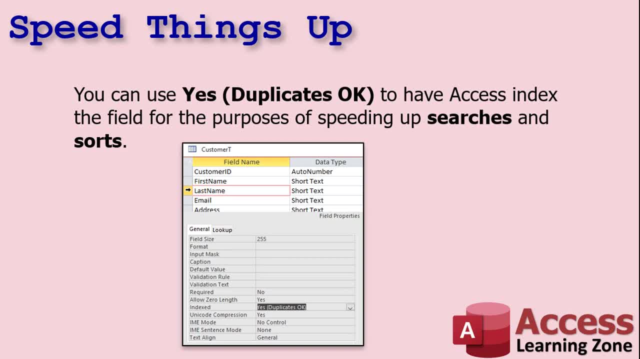 to have Access, index the field for the purposes of speeding up searches and sorts. For example, let's say you do a lot of searching on the customer based on their last name. You may want to index that field but allow duplicates. You still want to allow multiple Smiths, for example, or Kirks. 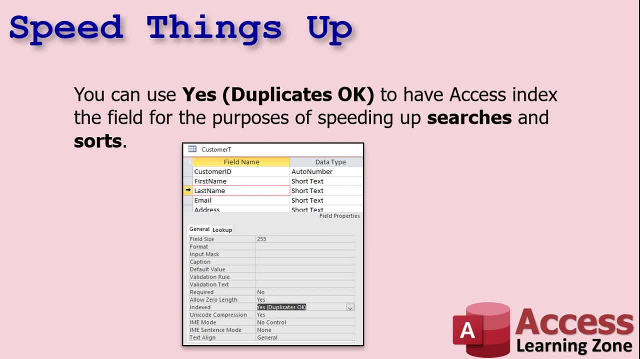 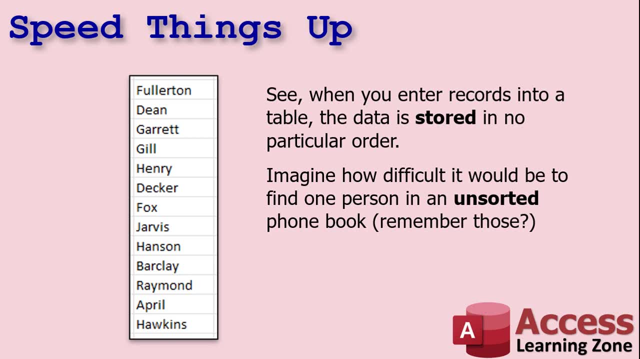 If you search on it a lot, if you sort on it a lot, you want to index it and duplicates are okay. See, when you enter records into a table, the data is stored in no particular order. So if you want to sort this list, it's slow. 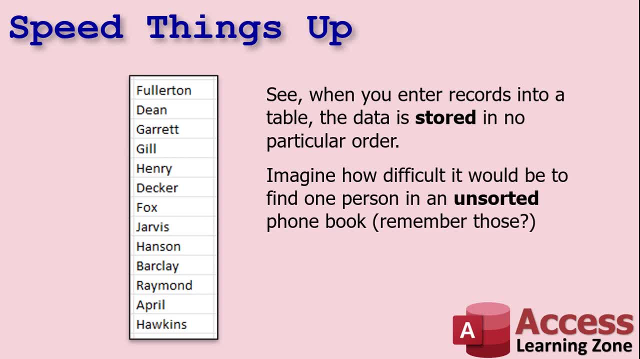 If you want to search for a single name, Access has to start at the top and run through all the records, one at a time, until it finds what you're looking for. Imagine how difficult it would be to find one person in an unsorted phone book. 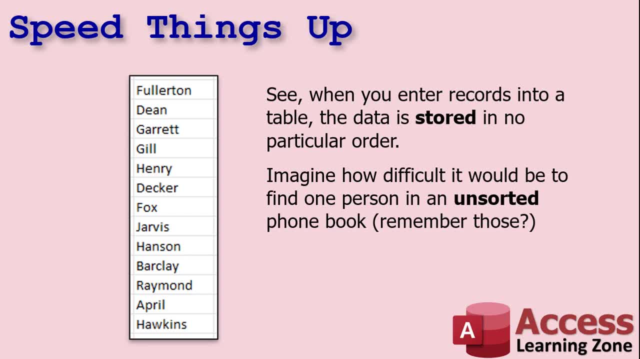 Remember those back in the day, Big, giant, thick books that the phone company would drop off at your house, Right, That's been a while. I haven't seen those out in a long time. Now I think they're just for businesses. 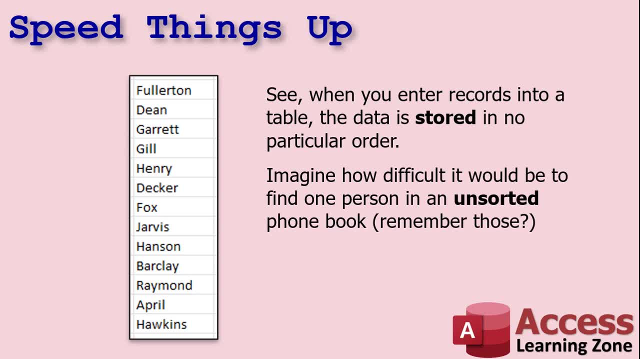 More of an advertising thing. But remember the phone book? right, I'm in the book, I'm old enough to remember that. Imagine trying to find a person in an unsorted phone book. That's basically what indexing does. So when you index a field, Access creates a separate index table. 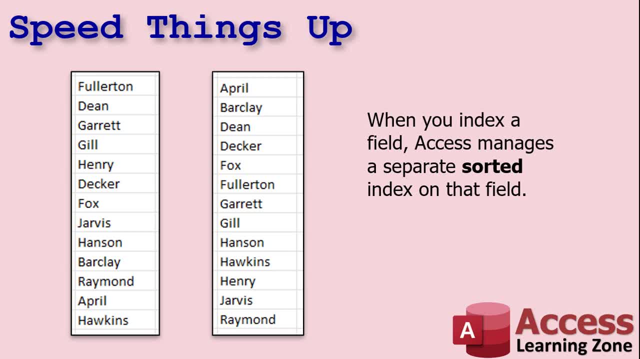 It's hidden. You don't see it. That it manages. It's sorted by that field and this greatly speeds up searches and sorts on that field. Access can use a faster algorithm and I'm not going to go into the details right now. 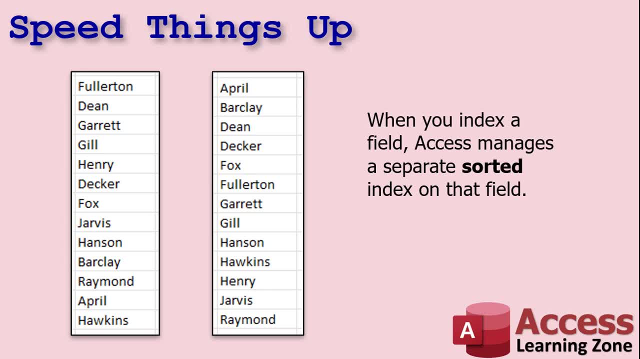 to quickly, to quickly, to quickly find a value in that sorted index. I have been thinking about doing some classes on computer science, which is the actual math and logic behind this stuff. So if you guys are interested in that, post a comment below. 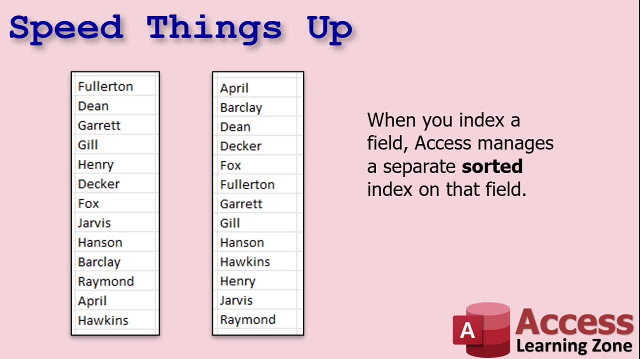 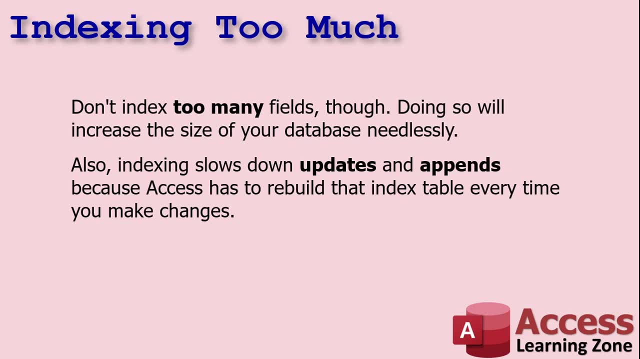 I took that stuff in college back in the 90s and it was pretty fascinating. Right, Different algorithms for sorting and stuff. Now you might ask: well, why don't I just index every field? Well, you don't want to index too many fields. 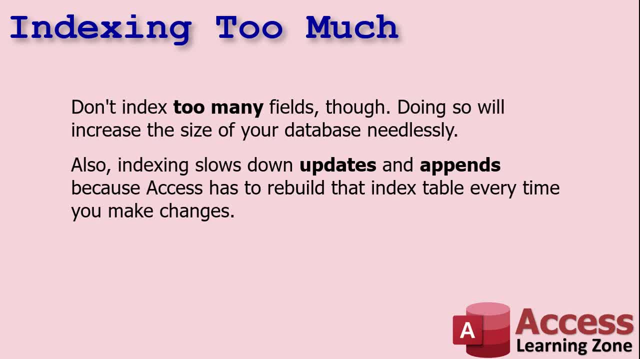 Doing so will increase the size of your database Needlessly. right. Every index table adds to the size of your database And indexing slows down updates and appends. right If you change or add records, Because Access has to rebuild that entire index table every time you make changes. 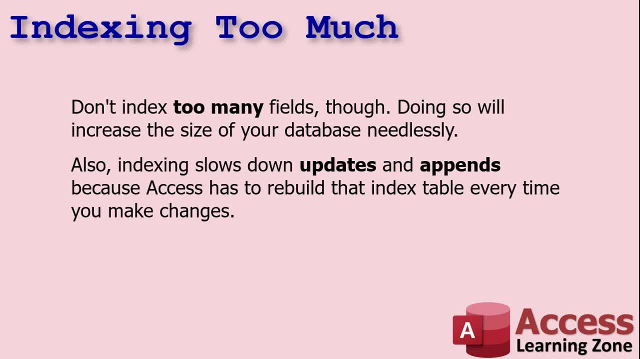 In fact, if you do more data entry and editing than lookups, you may want to consider not indexing your fields. If you've got a dozen people doing data entry all day long, like in a call center, and you only run a few fields, you might want to do more data entry. If you only run reports on that information once a month, go easy on the indexing. It's all situational, based on the needs of your business. If you do a lot of searches and sorts on a particular field and it's running slow, try indexing that field. 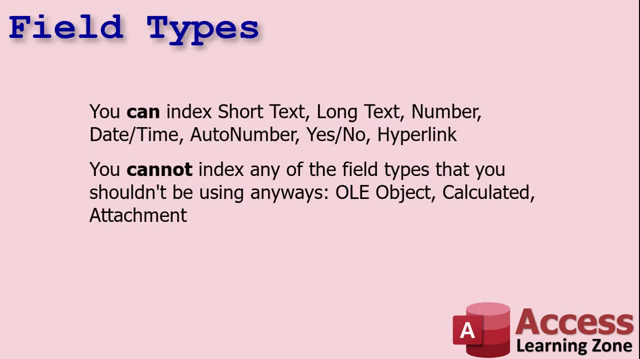 Alright, let's talk about field types. You can basically index every type of field that you should be using, although you might not always want to. You can index short text, long text, number, date, time, auto number, yes, no and hyperlink fields. 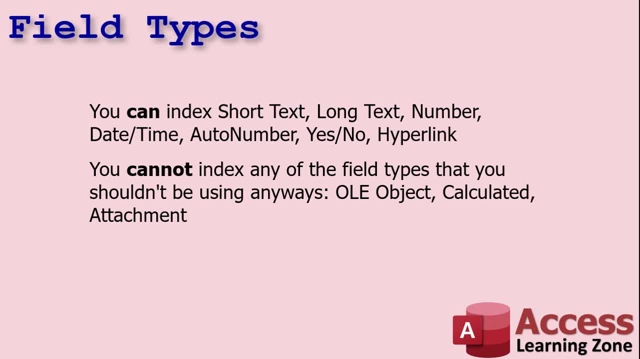 You cannot index all of the evil fields, All of the field types that you shouldn't be using anyway. OLE object: basically pictures and documents that get stored in the database. we don't do that. Calculated fields: we don't put calculated fields in our tables. we save that for queries. 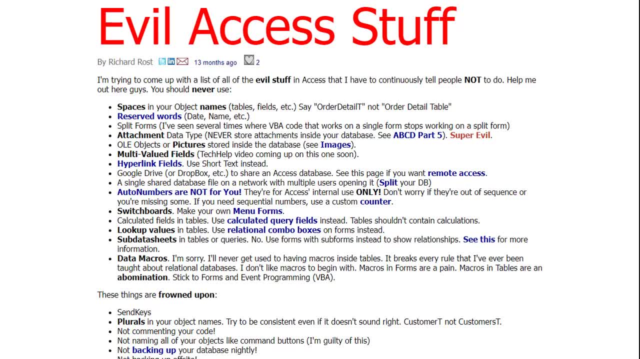 And attachments. again evil- Want to see all the evil access stuff. I've got a page for it. I'll put a link down below. you can click on and go read all this stuff. I'm going to make a video on this eventually. I'm still compiling it. 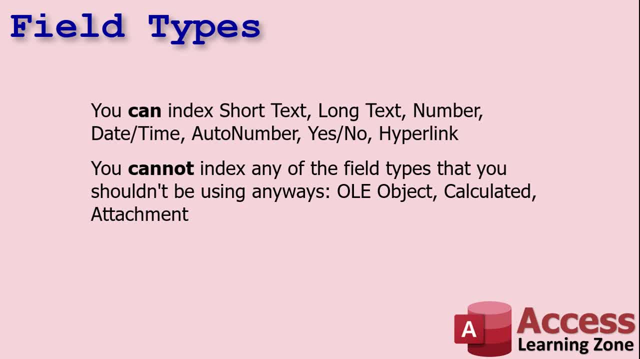 In older versions of access, you didn't used to be able to index memo fields, which are now long text fields, And in fact, if you're watching an older version of some of my lessons, I mentioned that you can't index memo fields. 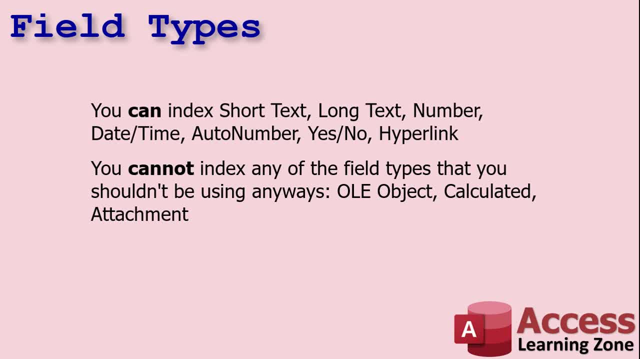 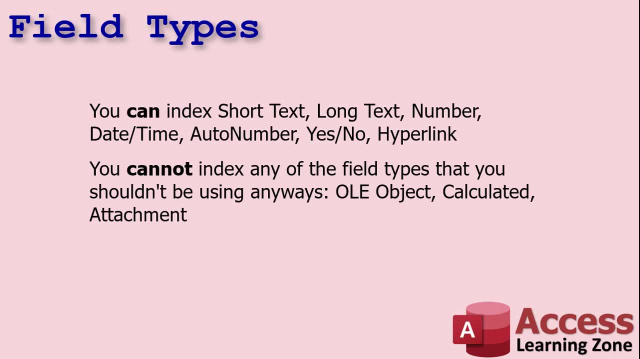 You can now, but I don't really see much of a point of doing that. It can really be a hit on the performance of your database. if you have indexed long text fields, So use those sparingly, OK, now here's a weird one. 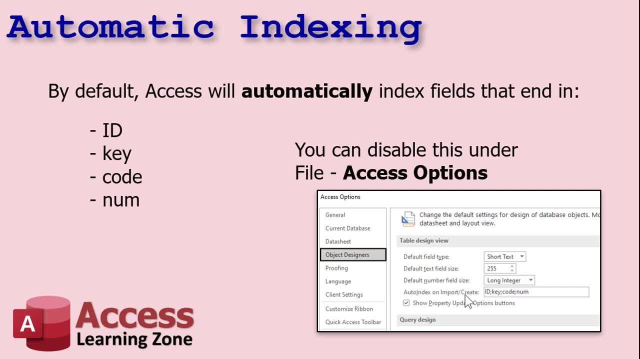 By default, access will automatically index fields that end in ID key code num. All right, those suffixes. So if you put a customer ID In a table, even as a foreign key, it's going to get indexed duplicates. 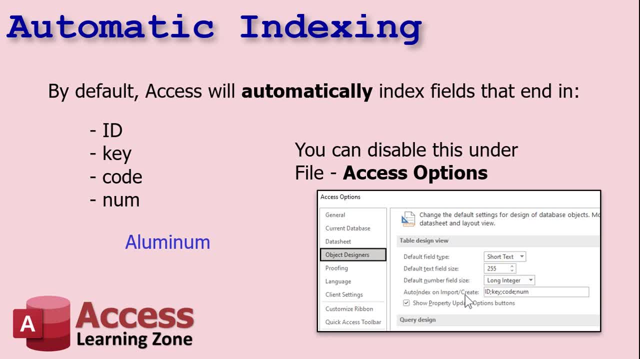 OK, But access will also index the word aluminum if it's a field, which I think is kind of silly. So if you don't like this, you can disable this under file access options. Go to object designers and you'll see auto index on import create. 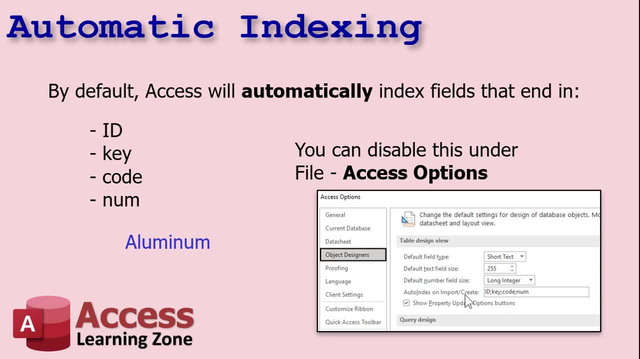 It'll turn these auto indexes on for these field types Anytime you create a new field or if you import it from something like Excel. OK, Just remove these options here. I usually leave ID in there, but like key code and num, I usually get rid of those. 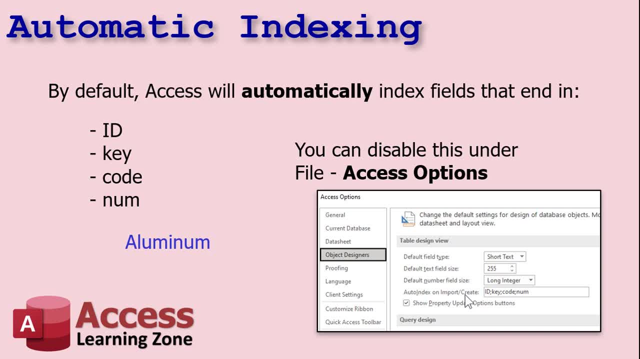 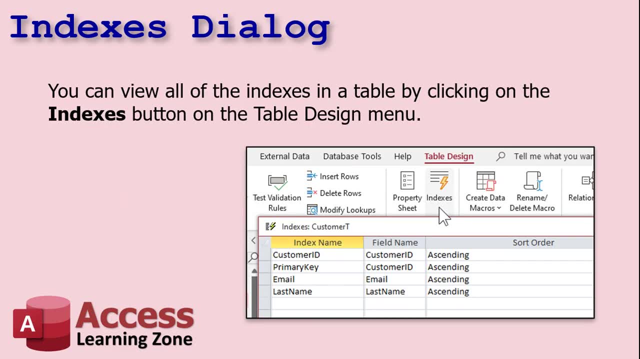 That's up to you. Will the extra indexes hurt? Yeah, probably not much. That's not going to probably hurt you that much, but it's just something to think about. OK, so there's an indexes dialog box. You can view all of the indexes in a table by clicking on the indexes button on the table design menu. 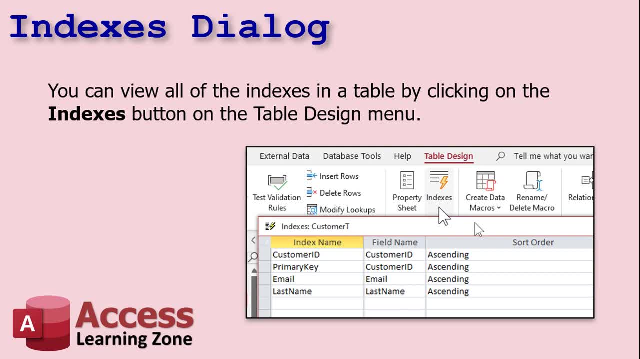 This little guy right there. It opens up this thing. Yeah, I know It's a little cut off picture of my screenshot In here. you can create something called a multi field index, which is rare, but I use them once in a while. 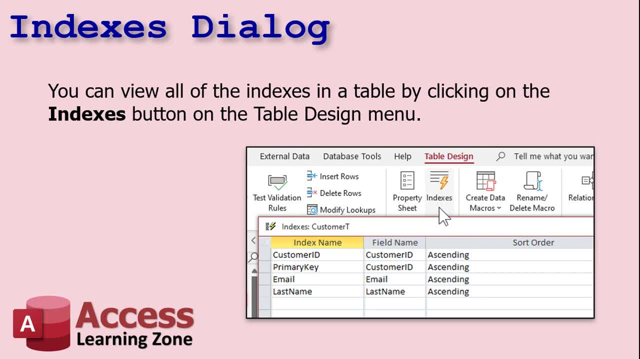 Let's say you routinely search or sort based on last name and first name together. Right, Smith Joe? for example, Creating a multi field index means that your database now has an index built containing these two fields together And it doesn't have to search through two separate index tables. 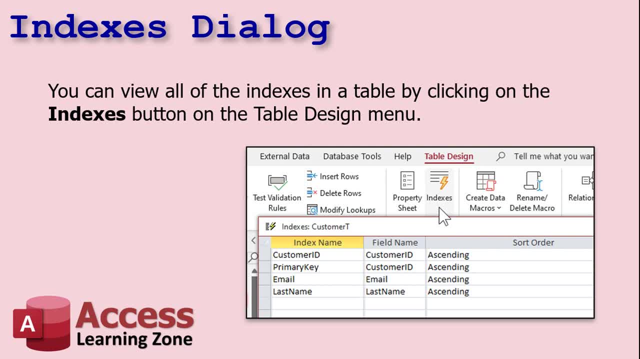 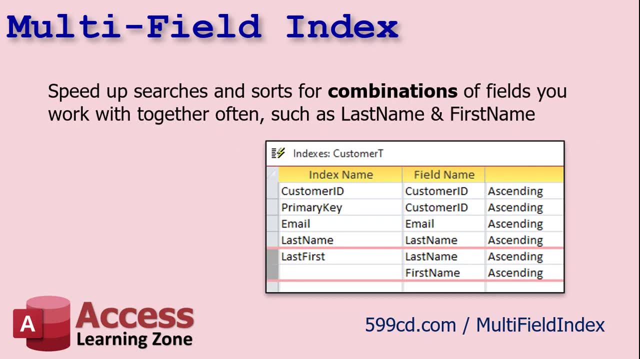 Again, this only really makes sense If you've got a zillion records In a huge database, but it can greatly improve performance if that's something you do a lot. I've got a separate video on building a multi field index and why you'd want to do that. 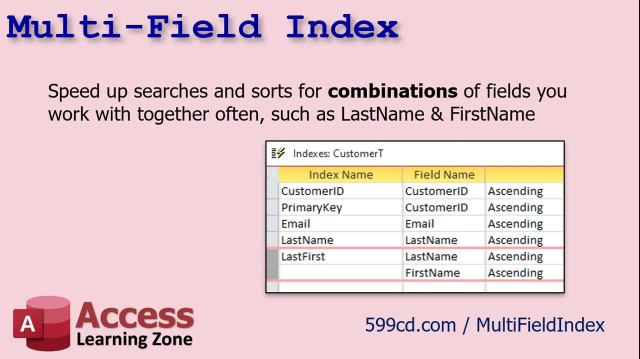 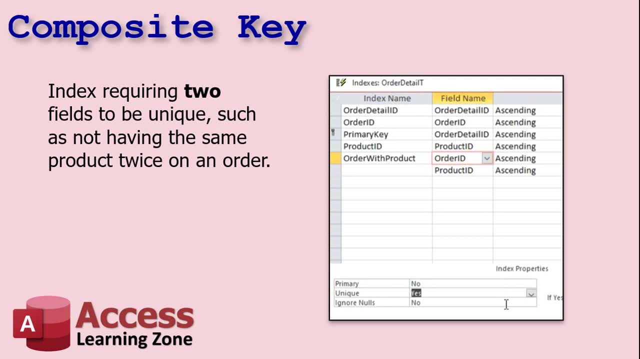 Check out that website for more Again. I'll put a link down below. You can click on it. Usually, the only time I'll set up a multi field index is when I'm creating something called a composite key. All right, That's an index requiring two fields in the table to have unique values. 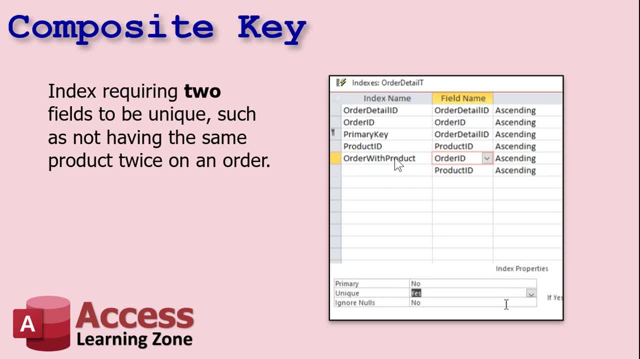 For example, here I create an index called order With product and it indexes order ID and product ID So you can't have the same product listed twice on one order. Those two things have to be unique: Right Order one product to order one product three and so on. 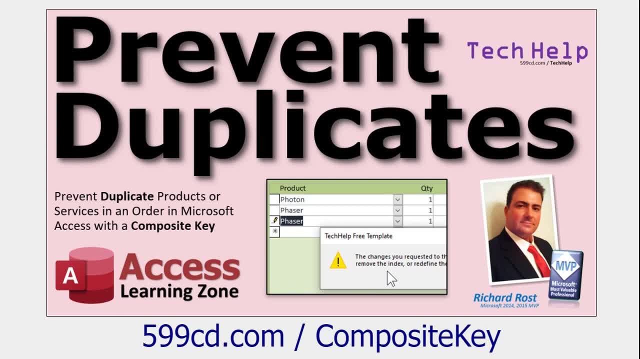 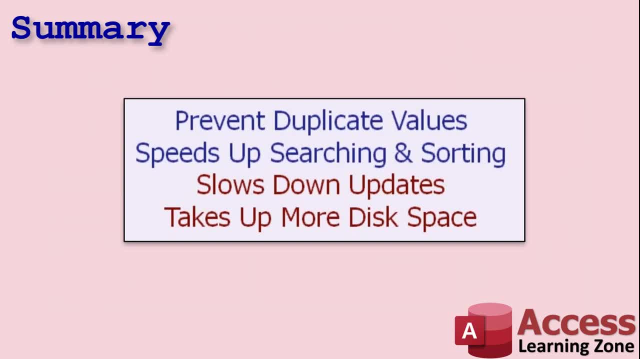 Again want to learn more about it. I got a video Here. you go Right, I'll put a link down below. So, in summary, indexing prevents duplicate values. All right. Customer ID, email address: whatever, And or. 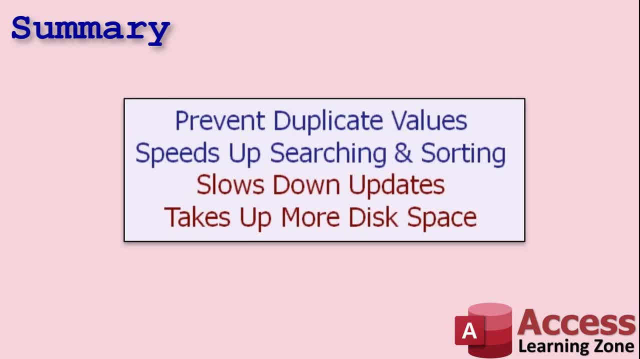 You can use it for speeding up searches and sorts. You can either make it unique. values or duplicates are okay, But on the downside you don't want to overuse them because it will slow down updates when you add or change records and it will take up more disk space. 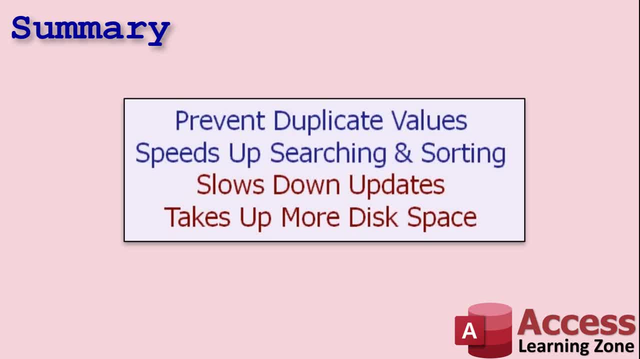 Now, to be completely honest, I usually hold off on indexing until I'm finished building my database. I don't try to think about it as I'm going ahead and working, because this is more of a performance issue, Unless you're dealing with the duplicate value thing. 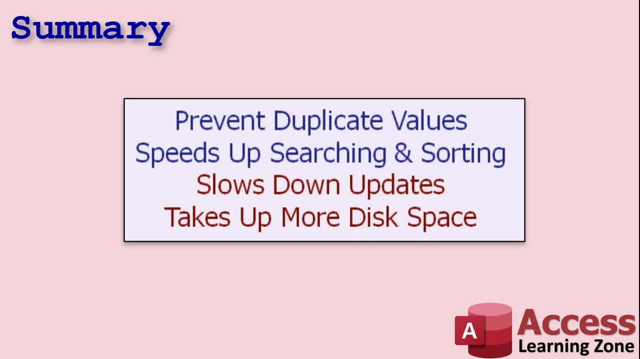 Like you want to prevent multiple phone numbers from being the same, for example. But as far as the performance issues go, that's something you can fine tune later. You can always add or remove indexes when your database is, you know, more mature and chugging along and you're wasting, you know, hundreds of megabytes of space. 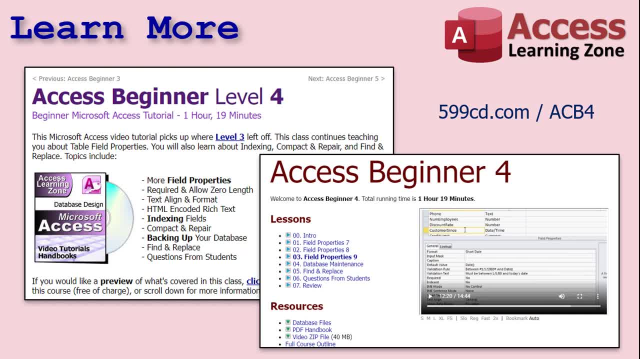 If you want to learn more about indexing, I cover it in my access. beginner level four, class. Yes, Beginner, I walk you through all the different fields in my database and explain which ones I index and why. we'll talk about each field and why you should or should not index it. 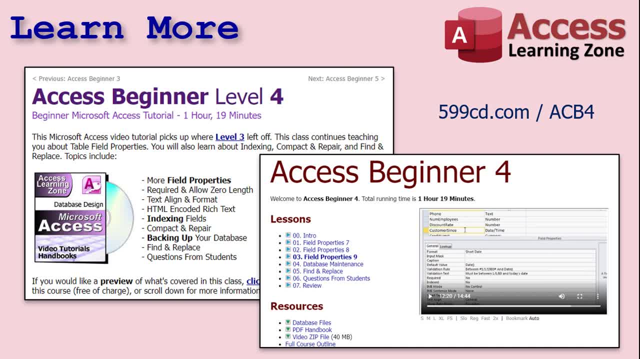 And this class also covers a lot of other field properties require it allows zero length, that kind of stuff We talk about compact and repair, backing up your database Lots more. It's an hour long class. You can find it on my website. 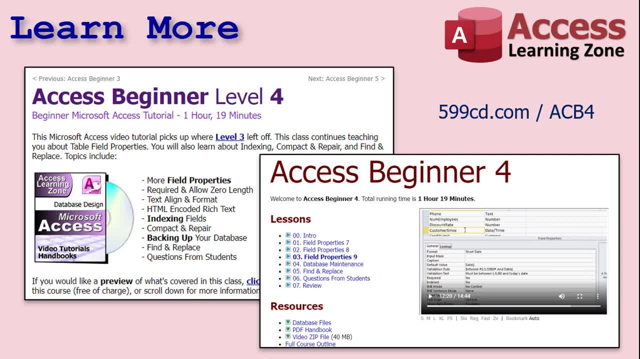 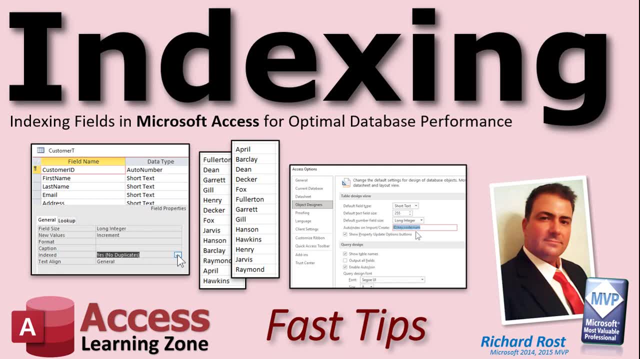 There's a link. I'll put it right down below Again, it's beginner level four. All right, So it's not an expensive one, And so there you go. There's your fast tip today about indexing. If you have any questions or comments, post them down below. 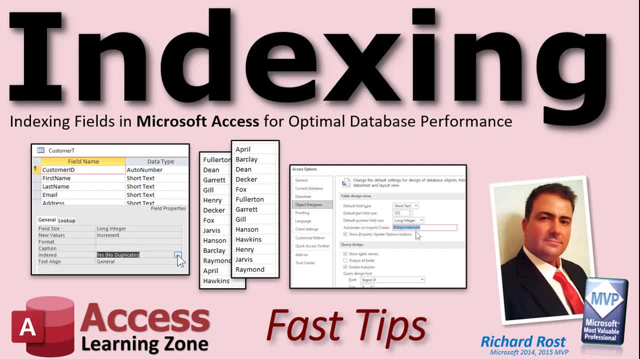 Hope you learned something I know I did. We'll see you next time. How do you become a member? Click on the join button below the video. After you click the join button, you'll see a list of all the different membership levels that are available, each with its own special perks. Silver members and up will get access to all of my extended cut tech help videos. One free beginner class each month and more. gold members get access to download all of the sample databases that I build in my tech help videos, Plus my code vault where I keep talking to you. 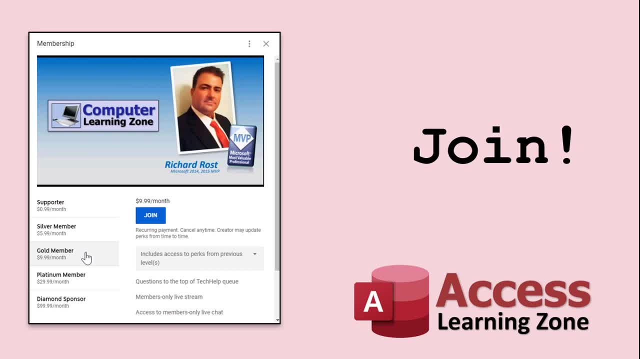 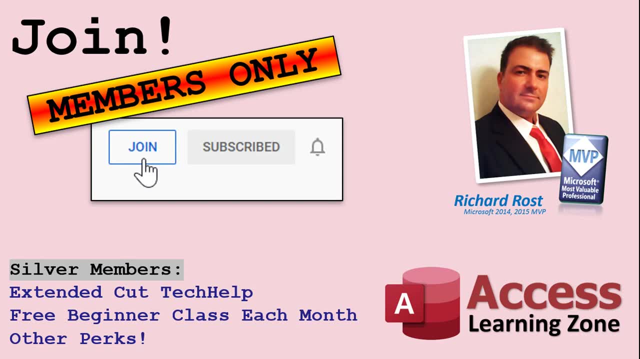 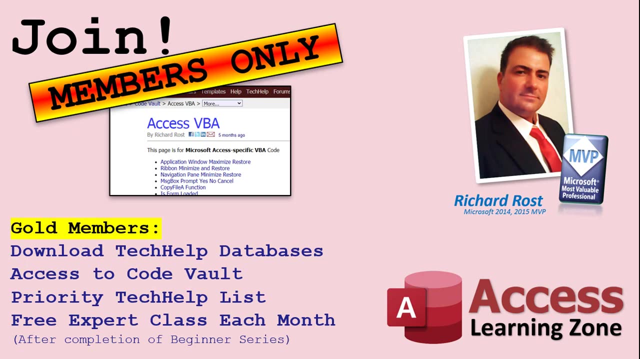 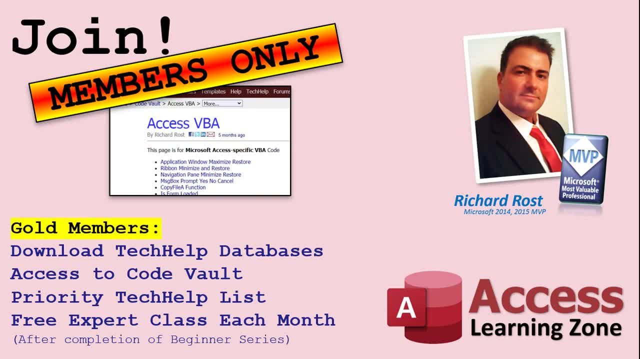 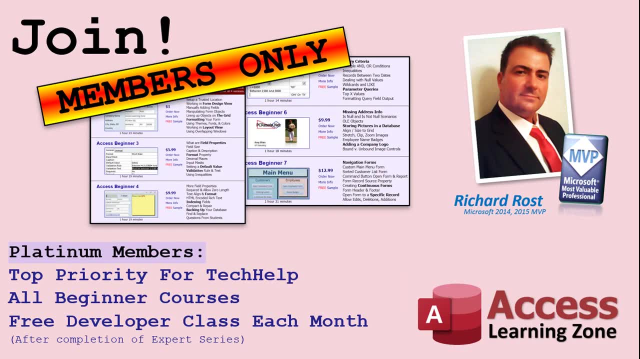